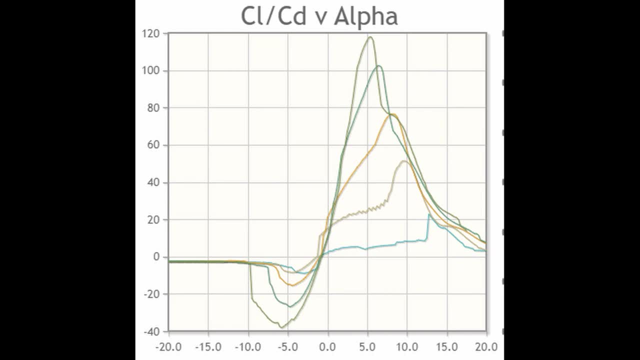 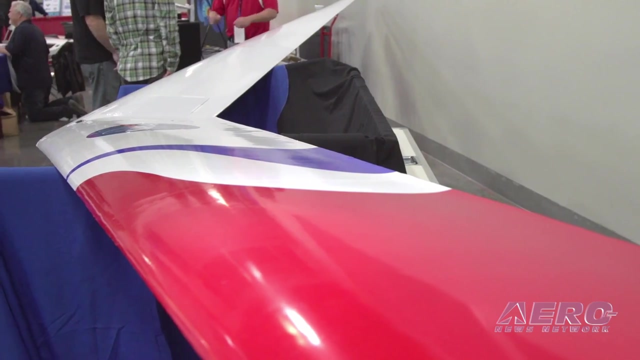 For the Reynolds number of cruising conditions. it has a maximum lift-to-drag ratio of approximately 75, at an angle of attack of about 5 degrees. The next step in the project consisted of determining other important factors of our wing design, such as the angle of attack, chord and wingspan of the airfoils. 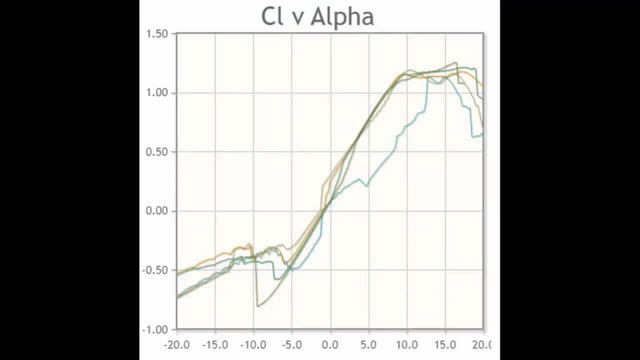 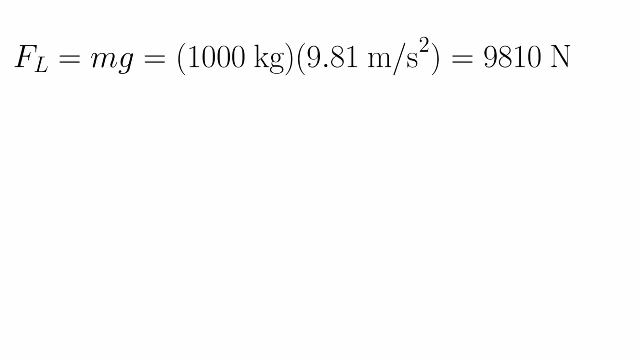 As seen in this graph, the Prandtl-D airfoil achieves the greatest lift coefficient, and therefore greatest lift, at a 10 degree angle of attack. This angle of attack will be used during takeoff to ensure maximum lift. The necessary lift force was then determined by using the equilibrium equation at takeoff. 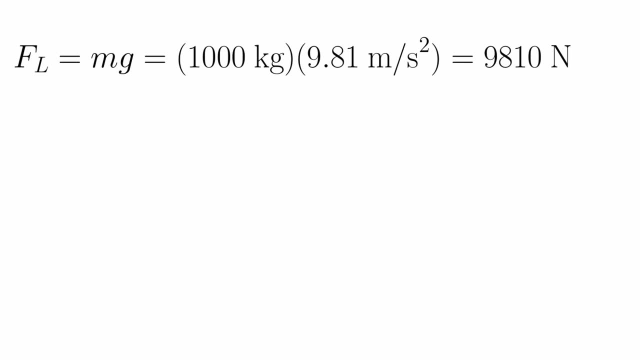 This equation states that the total lift force will be equal to the total downward weight force of the body. Therefore, it was determined that the total lift force necessary must be greater than 9810. N. Using the equation for the lift force, a necessary airfoil area was determined. 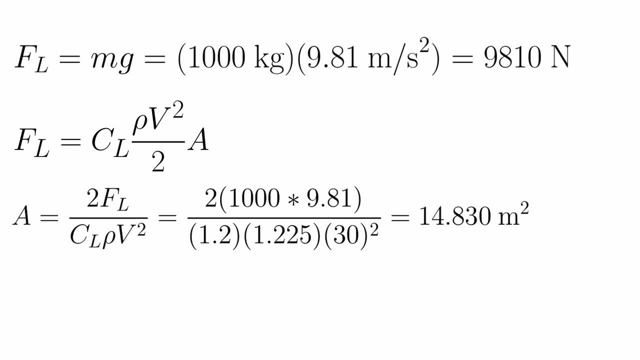 Because area is calculated as the product of airfoil chord to wingspan, one of these values needed to be assumed. in order to complete the calculation, A chord length of 1.5 m meters was assumed and using the calculated area of 14.83 meters, squared the wingspan. 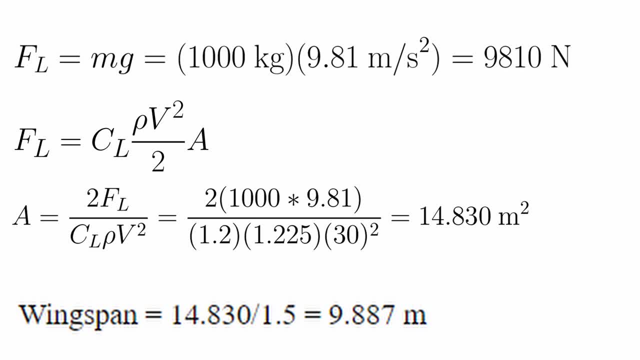 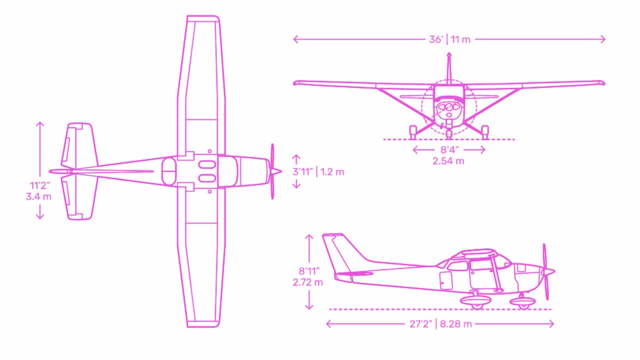 for the UAV was determined to be approximately 10 meters. This value was rounded up to 12 meters to allow for more leeway within the lift. This value is in accordance with the modeled Cessna 172,, which has a wingspan of approximately. 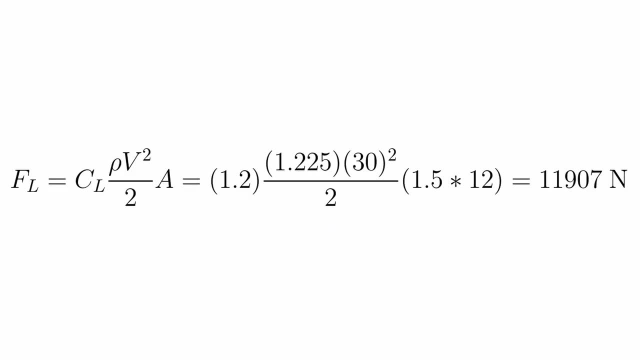 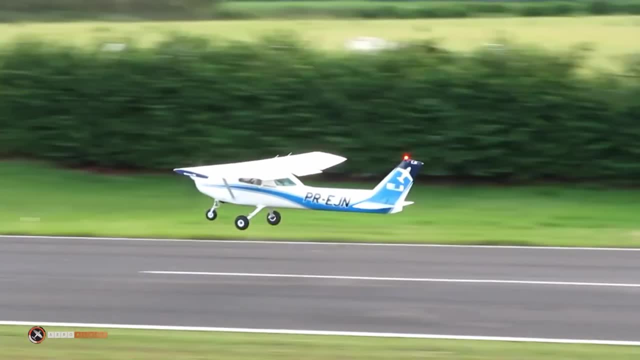 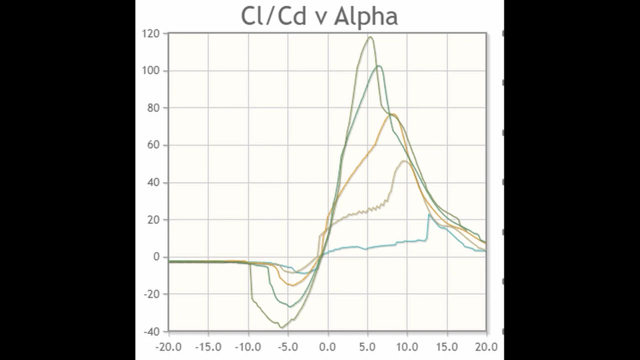 11 meters From here. the lift force during takeoff was calculated to be 11,907 newtons, which should be enough to get us off the ground. Now we need to calculate the drag, Looking back at the figure for the lift versus drag ratio compared to the angle of attack. 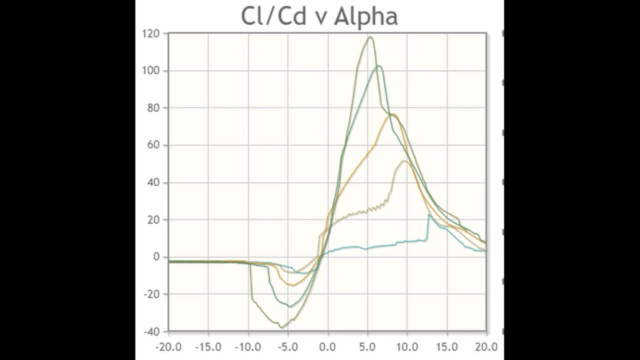 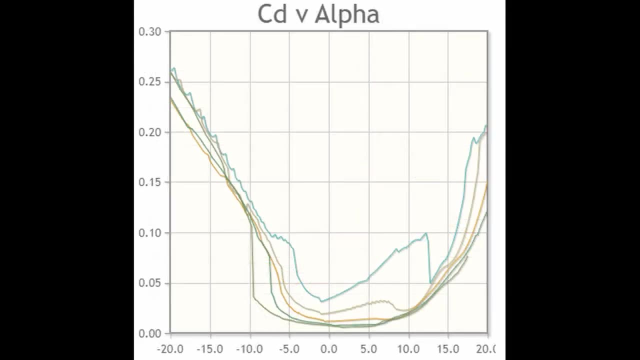 we can see that we can achieve the highest ratio at about a 5 degree angle of attack, which would mean that this would be our most efficient angle of attack to fly at Now. this graph shows the Prandtl-D's coefficient of drag values for any given angle of attack. 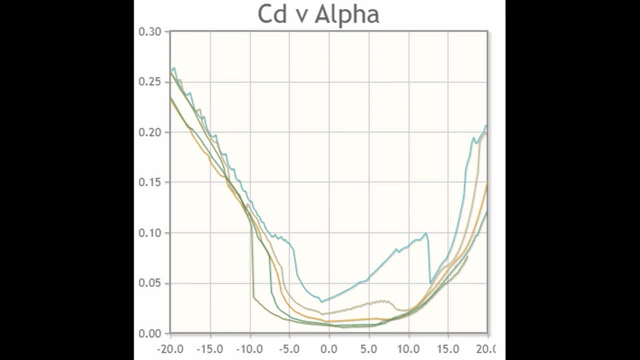 As you can see, the coefficient of drag is pretty low at the angle of attack of 5 degrees. Therefore, the angle of attack for 5 was chosen for the UAV's cruising conditions and the value for the coefficient of drag pulled from this graph. 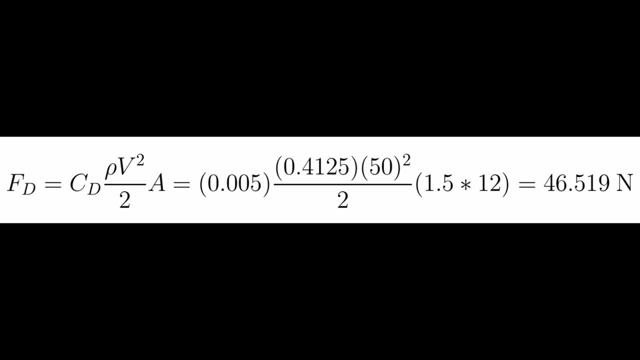 Using known values of the coefficient of drag velocity, air density and wing area during cruising, the drag force applied to the wings could be calculated at about 46.519 newtons. To quantify the drag acting on the fuselage of the vehicle, we need to calculate the drag. 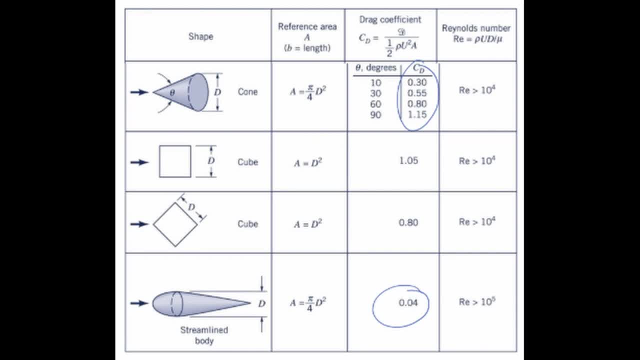 force applied to the wings at about 46.519 newtons. To quantify the drag acting on the fuselage of the vehicle, we need to calculate the drag force applied to the wings at about 46.519 newtons Since the measur naked temperature. Deutschen Hong groundwater 0.. grant oggi li. 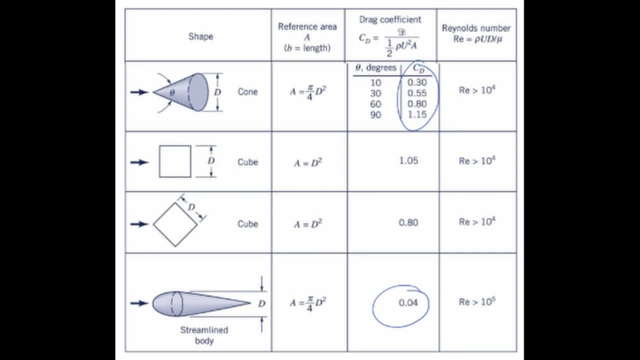 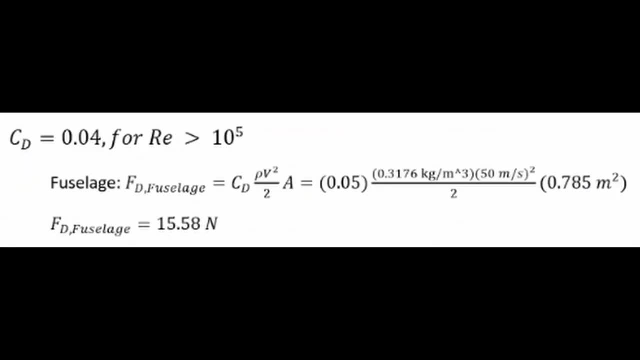 was assumed to be a streamlined by. since the calculated Reynolds, remember, was greater than the necessary value 10 to accept, the track of respective steam line body can be set at 0.04. the stalling was used to calculate total drag of the fuselage and it came up. 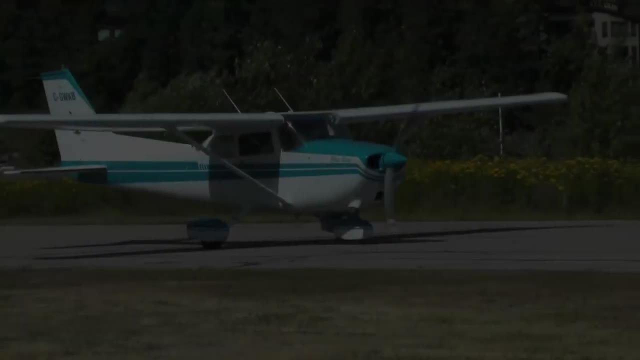 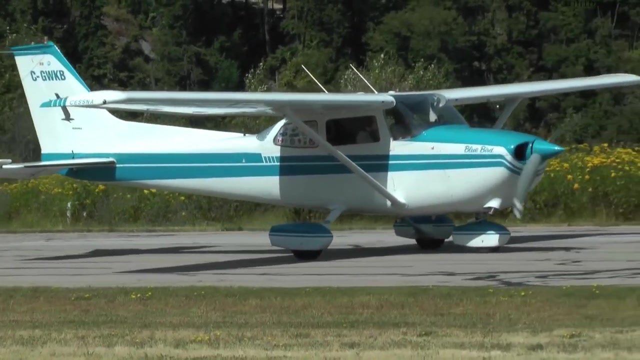 out to be about 5.6, 0, 1 use. next want to adjuvant stout requirement: propulsion estimate: dinner trap theаю. these three are was a log. the. The power of an aircraft is defined as the product between velocity and drag force. 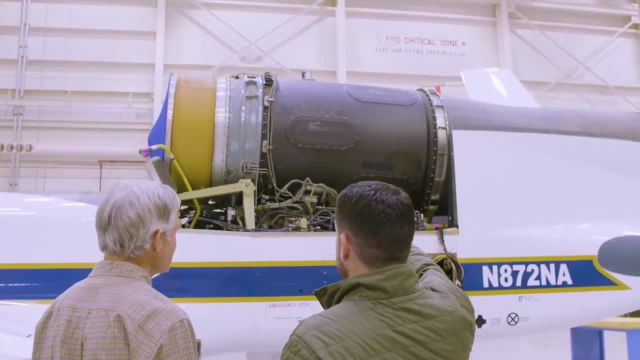 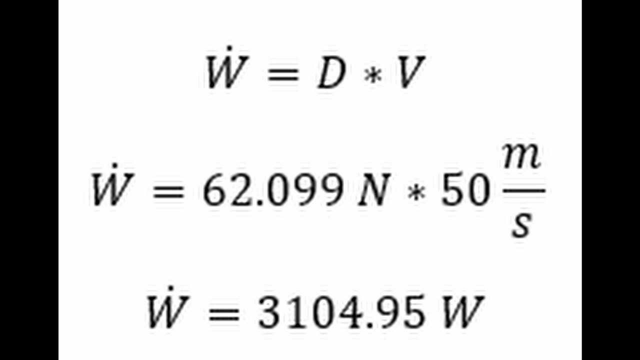 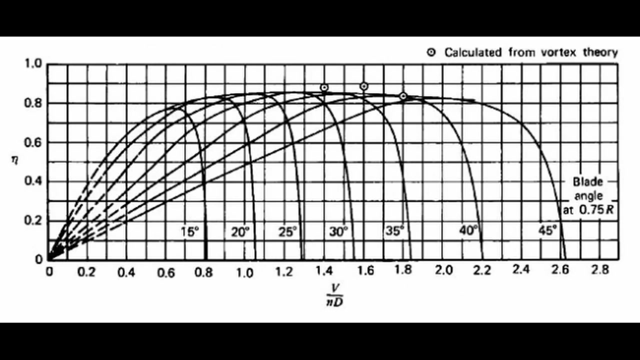 For this calculation, a summation of the drag force acting on the wings and the fuselage was required. The power at cruising conditions was determined to be 3104.95 watts. The selected propulsion method for our UAV was by propeller. After initial research, it was discovered that most propellers max out at an efficiency. 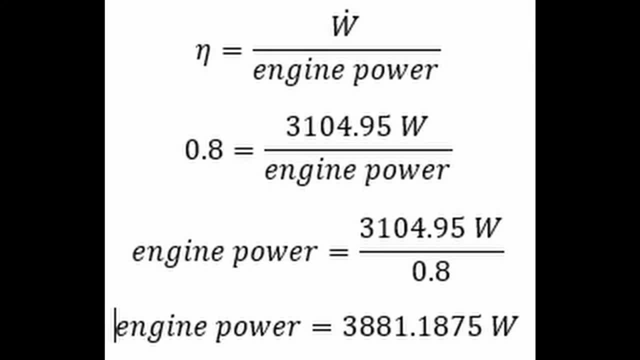 of about 0.8.. With this knowledge and with the determined power, the engine power was calculated to be 3,881.1875 watts, or an equivalent of 5.205 horsepower. Commercial engines that could achieve this horsepower were researched. 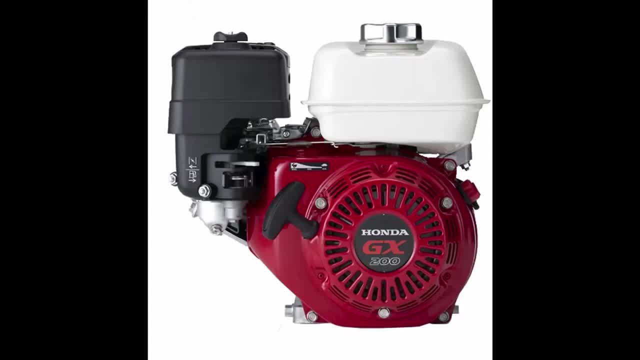 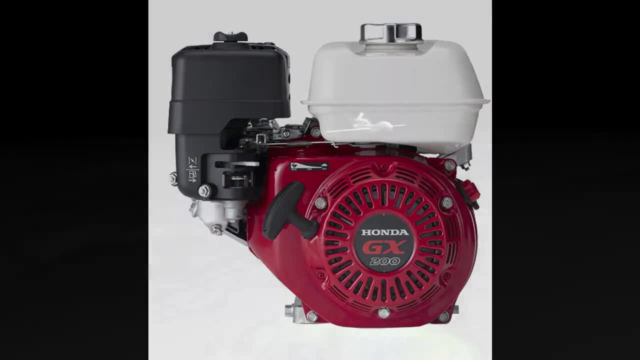 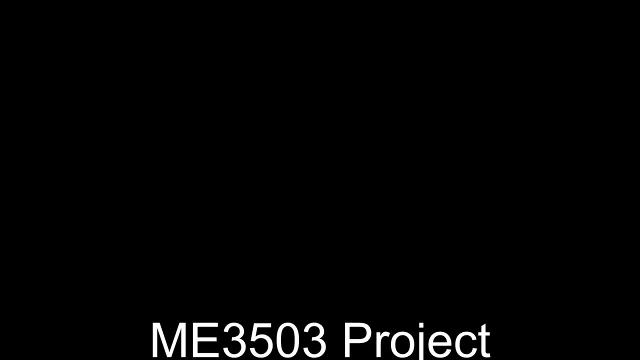 The team decided upon the Honda GX200,, which has a maximum horsepower of 5.5 horsepower. The specs for this engine include a fuel consumption rate of 1.7 liters per hour. The model's engine is a four-cylinder and the engine is equipped with a low displacement.